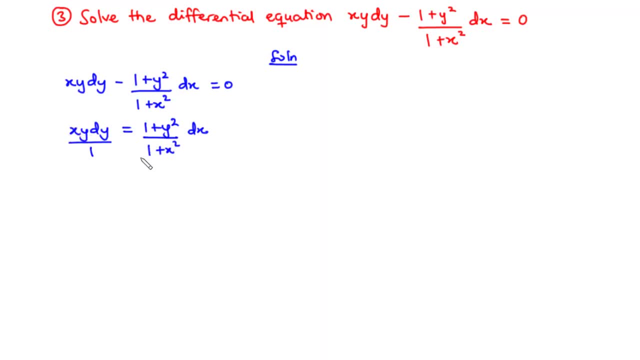 So we can pull x from this side to be a denominator here And then we can pull 1 plus y square also to become a denominator here. So we are going to have y dy divided by 1 plus y square And that will be equal to: we have 1 over x times 1 plus x square dx. 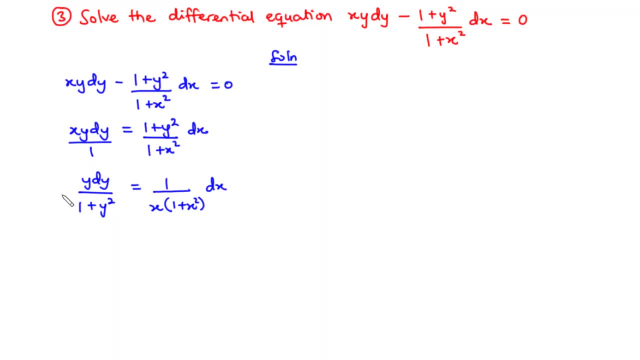 So here we've been able to group all y's on one side and then all x's also on the other side. At this point we can perform integration on both sides. Now from the left-hand side you realize that we have y dy over 1 plus y square. Now if we have something like 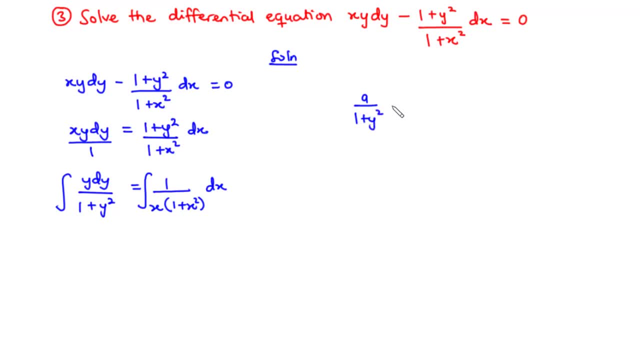 a over 1 plus y square dy, where a was a constant, we can represent that as a times 1 over 1 plus y square dy. And then you realize that if you want to integrate this, then this becomes: we pull out a and then we have ln of 1 plus. 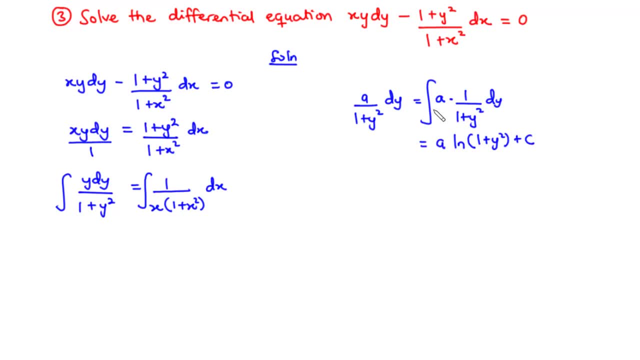 y square plus c. Now you realize that here is y, And so we can use this approach for integration, And so what we are going to do is to integrate this by u substitution. So by u substitution what we mean is we are going to represent part of this fraction by u. So 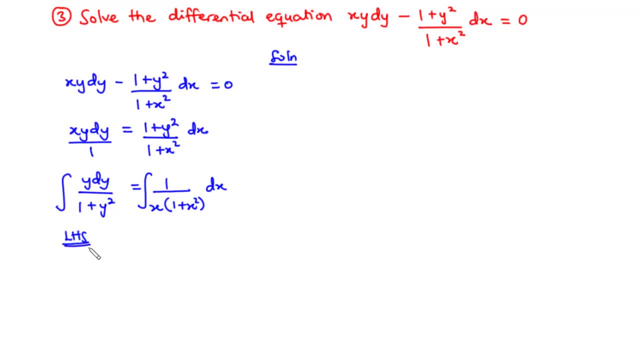 let's focus on the left hand side. So from the left hand side we have the integral of y y dy over 1 plus y square. So for this we can say: let u be equal to what we have as the denominator, So that becomes 1 plus y square, and then we can differentiate u with. 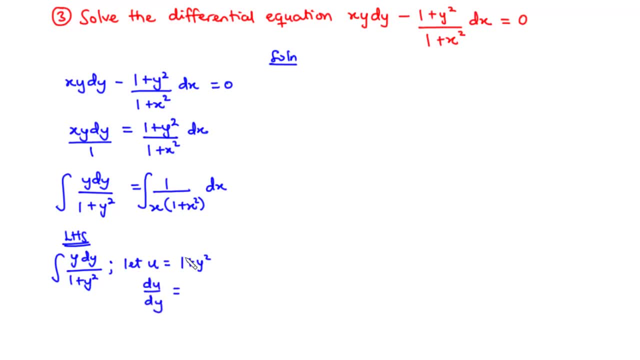 respect to y. Now, when you do that, you have this to be a constant, so it goes to 0.. You have this to be y square, so it becomes y. So this is 2x plus 2x times 2y, and then we want to make dy the subject, So we have dy. 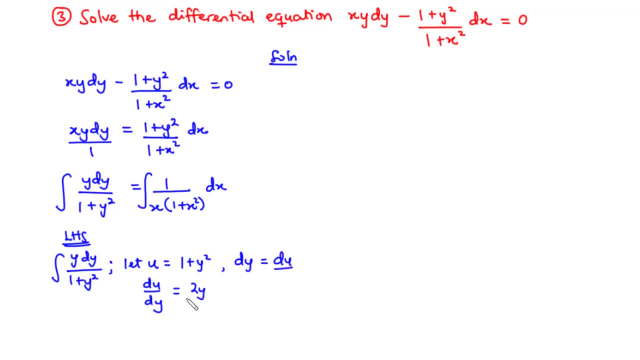 equal to. we just interchange the position of dy and then 2y so that becomes du divided by 2y. Now let's put dy and then u back into this, So you are going to have the integral of y timeswny divided by dy. 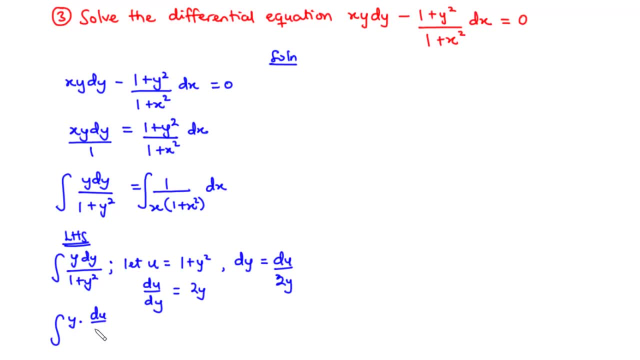 and that is du over 2y. all divided by u, this is u. so we cancel out y and then y, and then we are left with the integral of du over 2 times. now we are going to multiply that by the reciprocal of this, so u becomes 1 over u, so 1 over u. then we have this as: 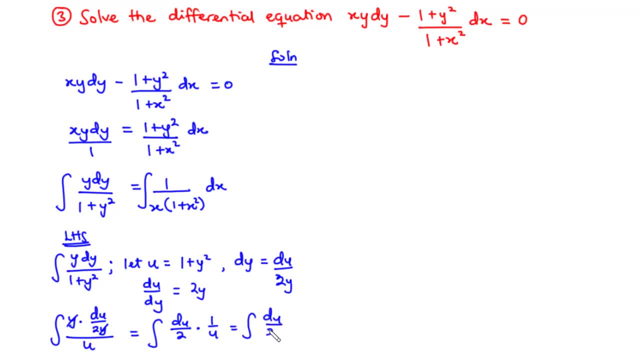 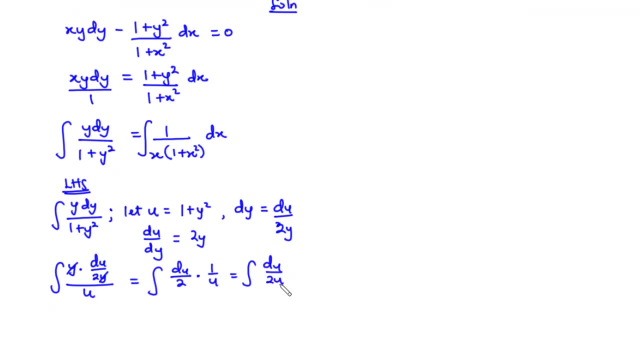 du over 2u. now we can think of this as 1 over 2 times du over u, so this becomes 1 over 2, so that, because that is a constant, you can pull out 1 over 2 and then you have the integral of du over u or, better still, 1 over u. 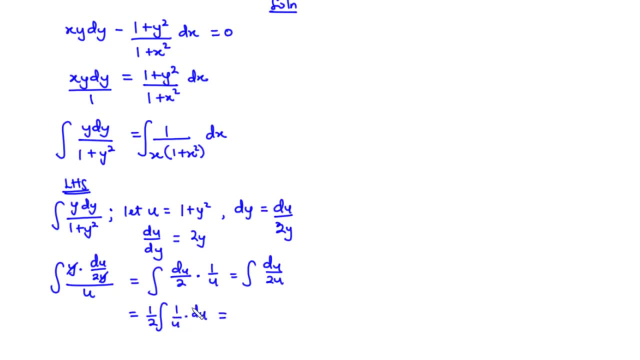 du over u and then we integrate 1 over u, so we have 1 over 2 times ln of u plus c. now we know that u is equal to 1 plus y square. so finally we have 1 over 2 times ln of 1 plus y square plus c. so that is only for the left hand side. 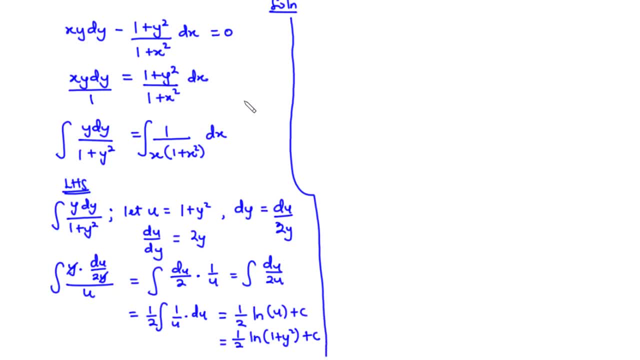 now let's move on to the right hand side. so also for the right hand side, we have the integral of 1 over x times 1 plus x squared dx. now here we have a linear factor of x, and then we have a quadratic factor of 1 plus. 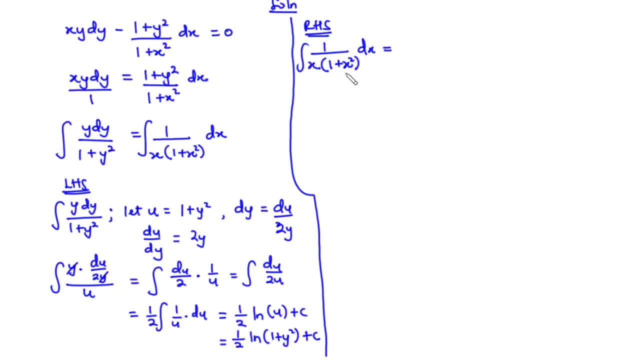 x squared, so we can think of integrating this by partial fractions. so we are going to separate this. now we are going to have a over the linear factor plus bx, plus c over the quadratic factor. so now let's try to solve this. so we have the lcm to be x times u squared by the rusty. 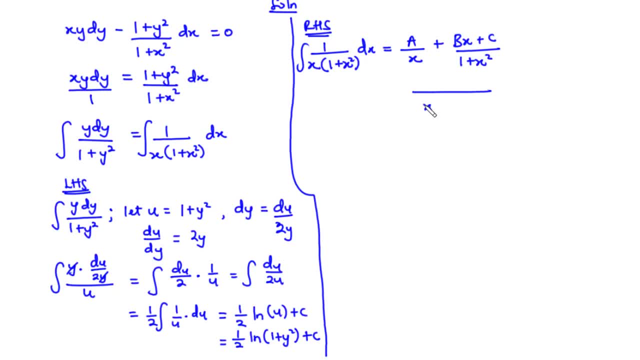 wave. and then we have thelling factor and it can be written down as this to solve this problem. so we have the lcm to be x times u squared. u squared over u taking u squared. here we have a chi力 factor: x times 1 plus x square. now, x times 1 plus x square, divided by x. x cancels out x, we are left. 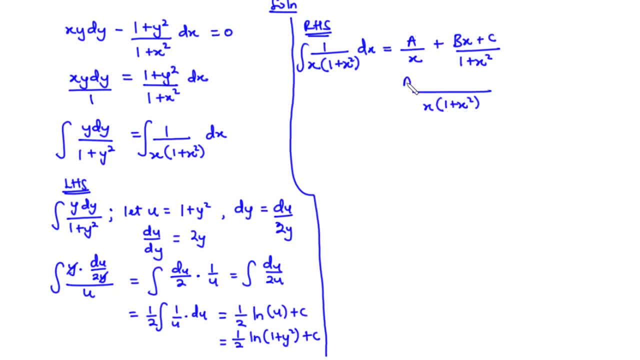 with 1 plus x square multiplying e. so we have e times 1 plus x square, plus this divided by 1 plus x square. this cancels out this. we are left with x, so times x, sorry, plus x. times bx plus c. so let's try to expand the numerator so we are going to have a times 1, that is a. 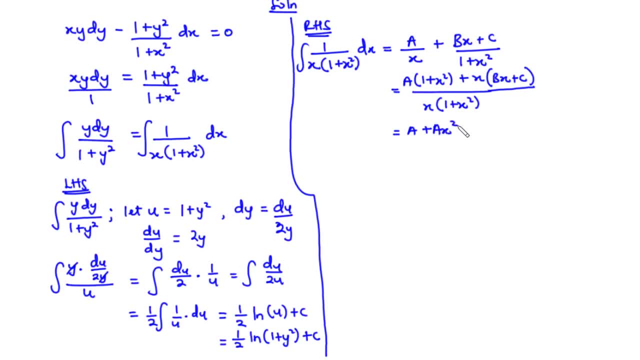 and then plus a x square plus b x square plus c x, we have a plus cx, plus we factor out x square, and then we have a plus b, a plus b. so that should be equal to 1. okay, that should be equal to 1. now, at this point, what we are going to do is we are going to 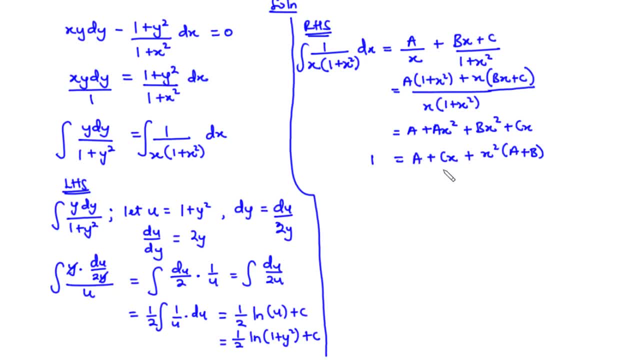 compare the coefficients of the constant times with x power 1 and then times with x power 2. so we are going to compare coefficients of the constant, the constant times of x power 1 and then x power 2. so let's start off with the constant. 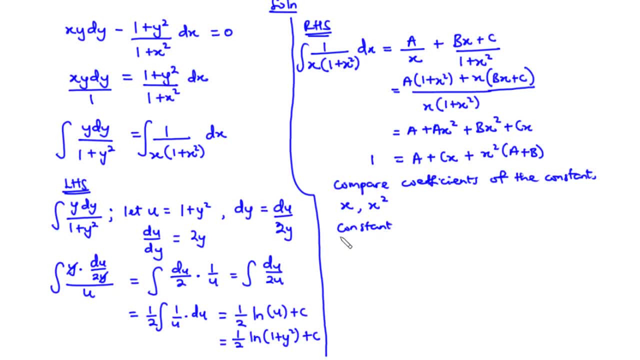 let's start off with the constant. so we have the constant on the left hand side to be 1. so basically, 1 is equal to a. so we have a to be equal to 1. now let's compare terms with power. with x, power, 1, we have only c. and then here we don't. 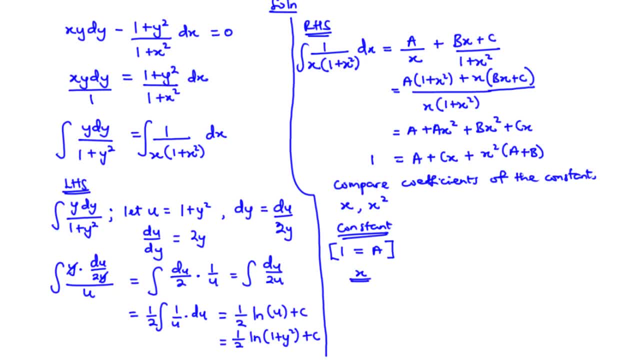 have any value with coefficients x, and so that's equal to 0. so it means we have c loss to be equal to zero. now we move on to x power 2. here we have a plus b, and that will be equal to 2, and then for this we have z plus z, square plus x, square plus b. x is equal to green minus w тоaya in. 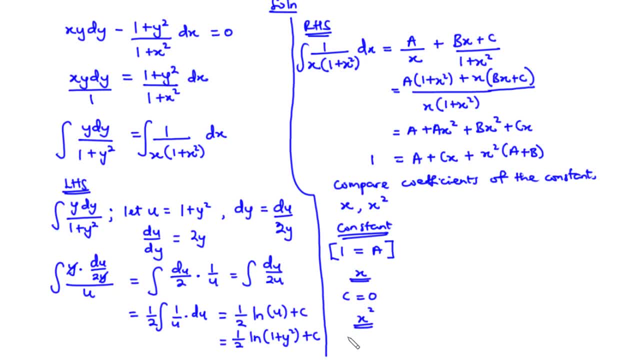 equal to 0 on the left hand side. So a plus b is equal to 0.. Now we have a to be 1.. So we can rewrite that as: 1 plus b equals 0, and then we have b to be equal to negative 1.. 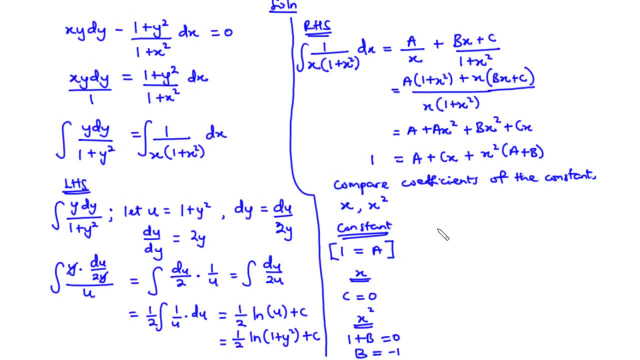 So what this primarily means is that we are going to have the integral of 1 over x times 1 plus x square dx to be equal to. we have the integral of. we are going to use this, So we have a to be 1.. So we have 1 over x, and then b is negative, 1. So minus negative. 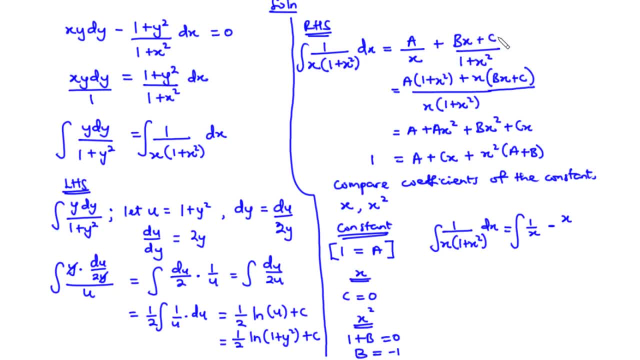 1 times x is negative x And then plus 0. So it still means negative x divided by 1 plus x, square All times dx. We separate this as integral of 1 over x. dx minus x over sorry, minus the integral of minus the integral. 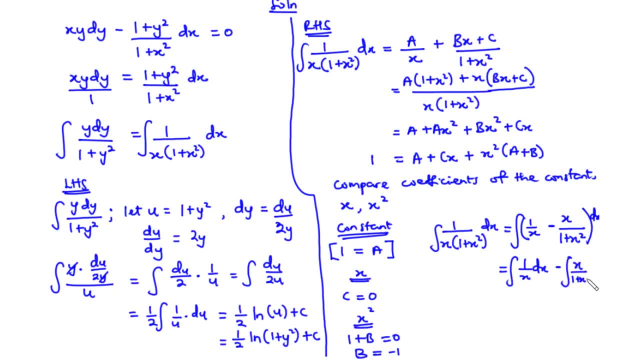 of x over 1 plus x square dx. Now let's try to integrate each of them. So when we integrate 1 over x dx now, you are going to have ln of x plus c And then, where you want to integrate this, what we have on. 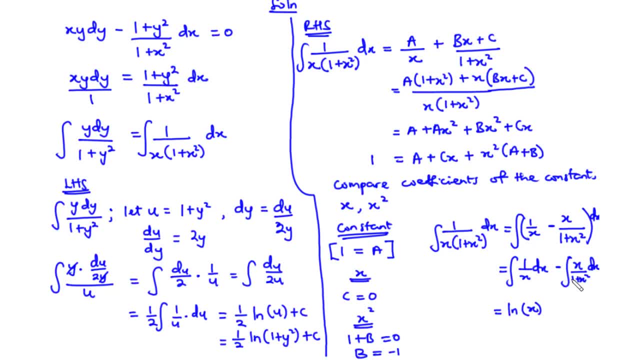 the right hand side, that is the integral of x over 1 plus x square dx. Now you realize that this is actually the same as integrating this, only that here we have x and the integral of x. So there are some aromaticities about this. That is the because the integral of x over 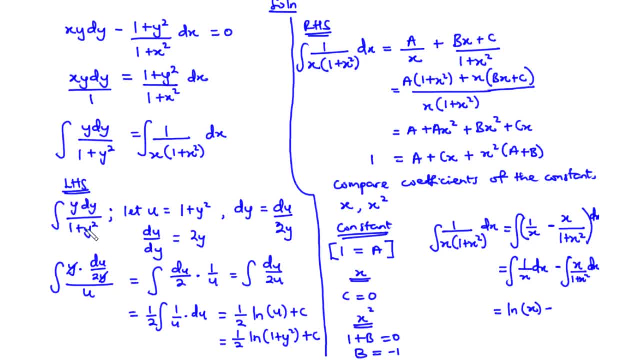 1 over x. what does that have in common with this? That is why we integrate this using the nth factor. So since the x particle is going to be that minus 1, then 1 is going to be 1 over x. Now. 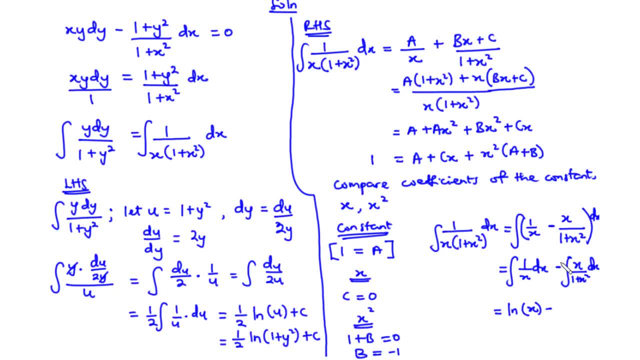 all these, we save this and we lower this removed. so we have an installation of x slash theס moved in economic range. we have x and then here we have y. now, when you do the same for x over 1 plus x, squared x, then 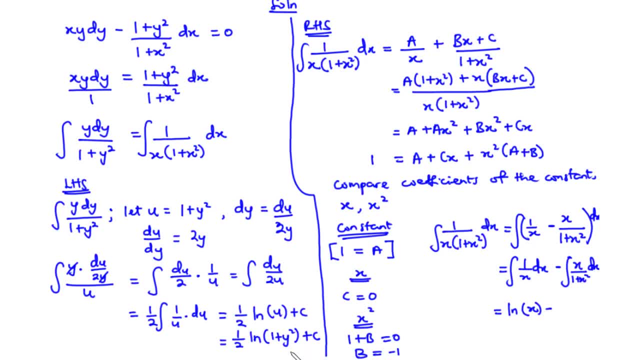 you are going to obtain this expression, just that here will be x squared, so that would be, let's say, ln of x, so that would be ln of x minus because of this negative, so minus 1 over 2, ln of 1 plus x squared plus c. so that is what we are going to get after integrating this whole thing. 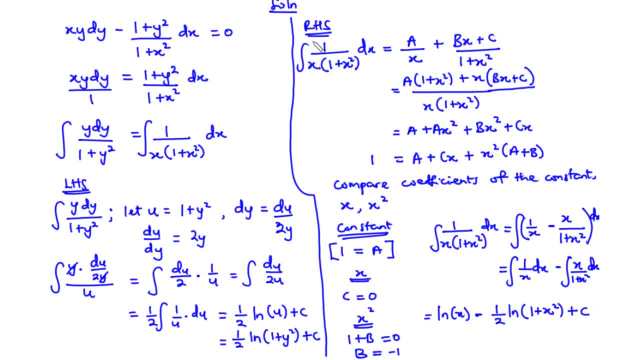 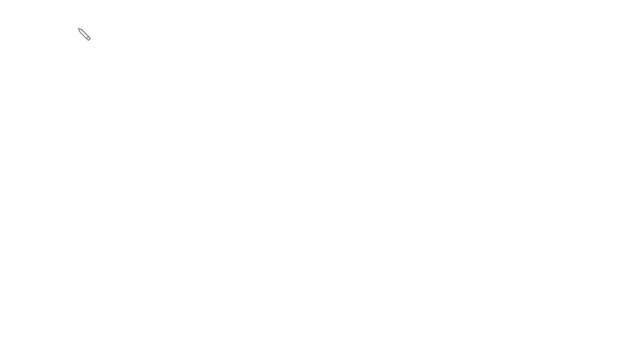 so this whole thing is also for only the right hand side. now in the next section we are going to equate the left hand side to the right hand side. so we are going to have 1 over 2, 1 over 2, ln of 1 plus y squared. now we are going to ignore the constant. 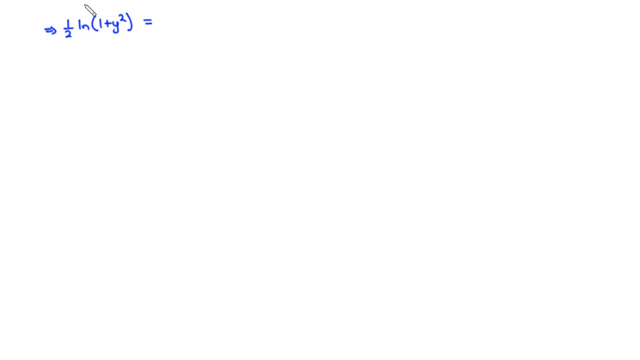 and that is equal to the right hand side. so this is the left hand side. that is equal to the right hand side. ln of x minus 1 over 2. ln of 1 plus x squared plus c. now let's transpose these terms: ln of x. 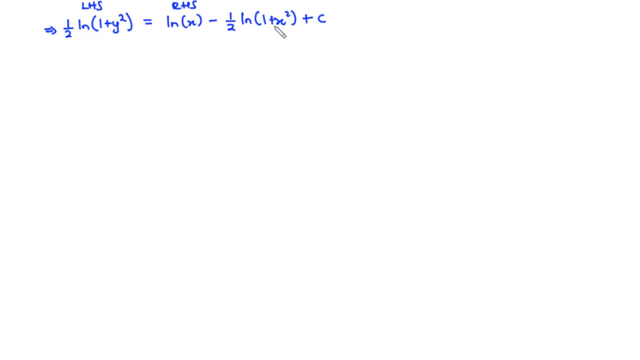 plus c and then negative 1 power 2 lm of 1 plus x square to the left hand side. so we have 1 over 2 ln of 1 plus preview of 2 ln of 1 plus x squares, minus ln of x plus 1. продолжăt x 1 over 2ln of há. 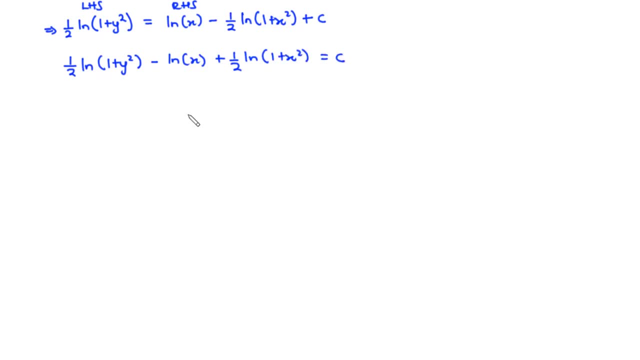 plus x squared, which comesность c. Now we can also represent another von Klier measure that is equal to 상tma 수, which is 2sizmiósormian. this as ln of 1 plus y squared, exponent 1 over 2, because this is the natural log. so 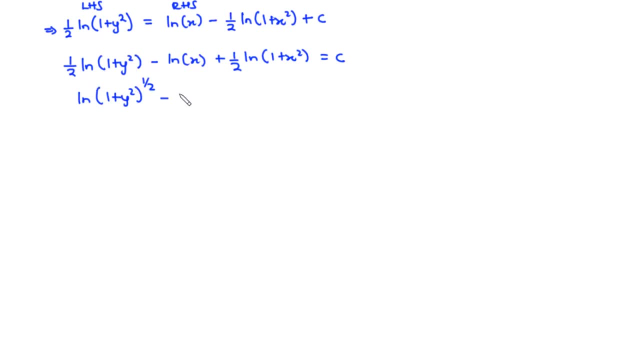 we can represent this as that, and so minus ln of x and then plus ln of 1, plus x squared exponent 1 over 2. now let's try to compress all these terms as one log. so we are going to have ln of, because this is negative, it's going to be divided. this is positive, it's going to be. 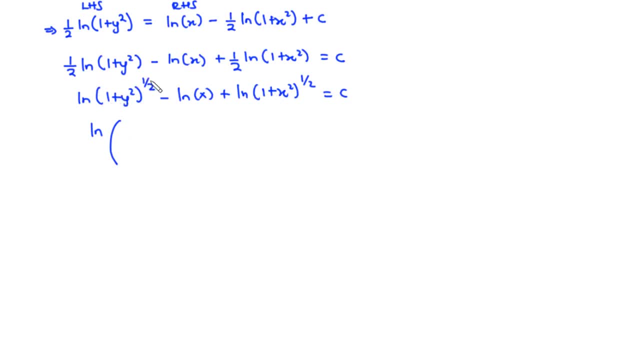 multiplying this and then, since we have to, the exponent 1 over 2, it means we are going to have the square root of this and then that, so it's going to be the square root of ln, of the square root of 1 plus y squared. 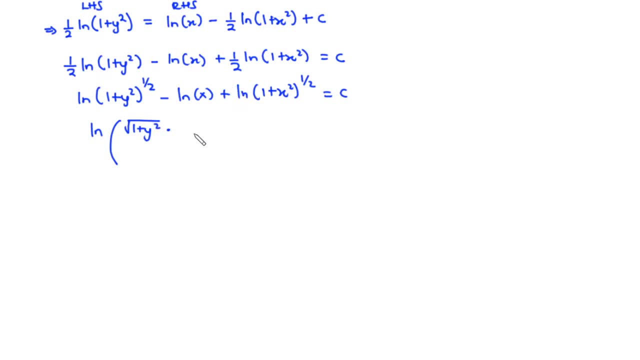 times, because it is we are adding, so we are going to multiply the square root of 1 plus x squared, and because we are subtracting, this is going to be dividing, and so we are going to have divided by, or divided by, x, and that is equal to c. now the natural log ln has a base of e. 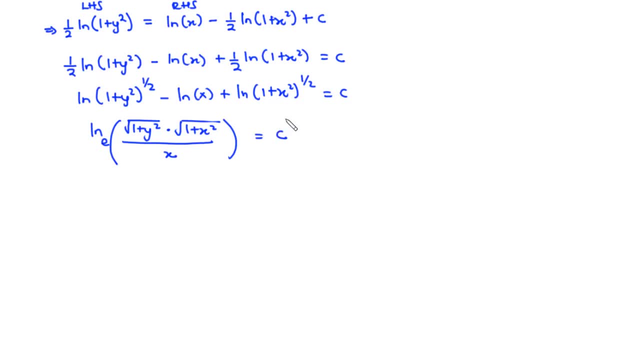 so let's bring that here. now we are going to transport c to be exponent on e, and then we equate it to what we have here, so that's going to be e to the power c equals. we have the square root of 1 plus y squared times, square root of 1 plus x squared. 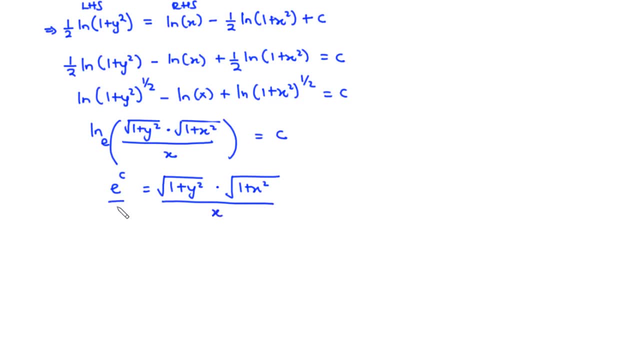 all divided by x. now let's cross, multiply, so we have x times e to the power. c equals square root of 1 plus y squared times 1 plus x squared. now, e is a constant and then c is also a constant, so a constant raised to the 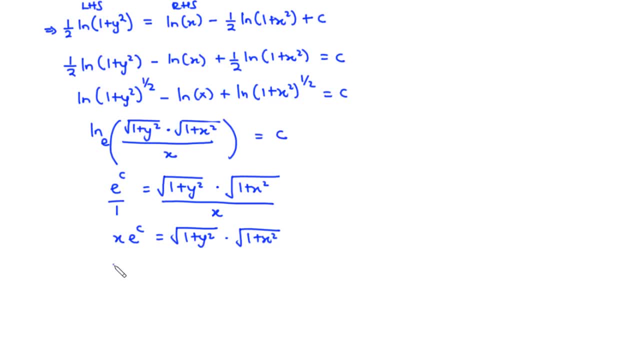 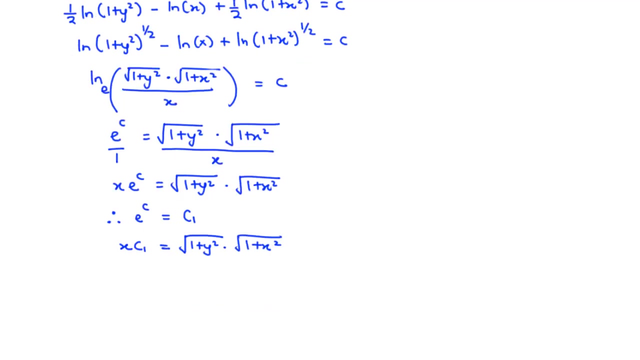 power. a constant is still a constant. therefore, e to the power c is equal to, let's say, c1, so that we simplify the equation: to have x times c1 equals square root of 1 plus y squared times square root of 1 plus x squared. now let's proceed. we should realize that we want to solve the. 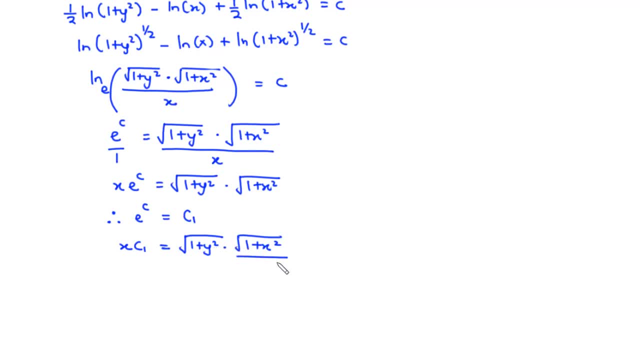 equation for y. so in this case we want to divide through by the square root of 1 plus x squared. so we divide through by the square root of 1 plus x squared. this cancels out that, and then we are left with x c1 over square root of 1 plus x squared. 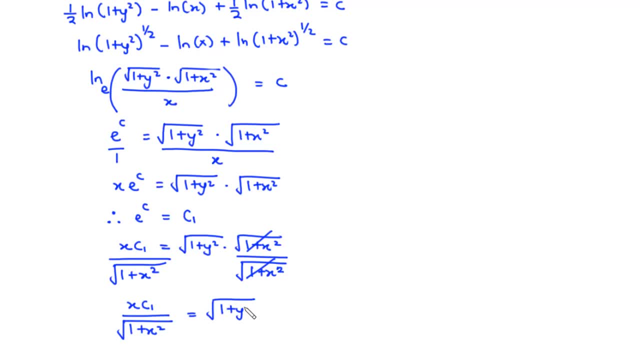 equals square root of 1 plus y squared. now we square both sides. we square both sides so the square cancels the square roots on the right hand side, so that we have 1 plus y squared and that will be equal to. here we are going to have x squared, c1 squared. 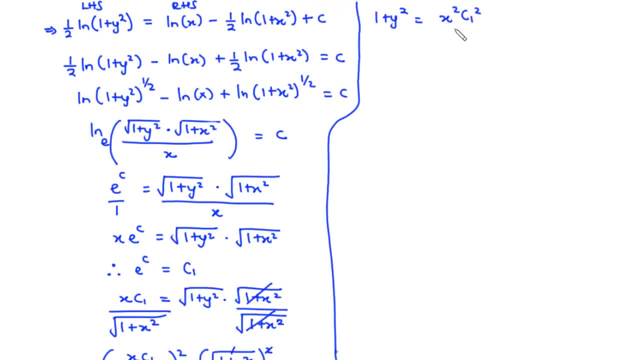 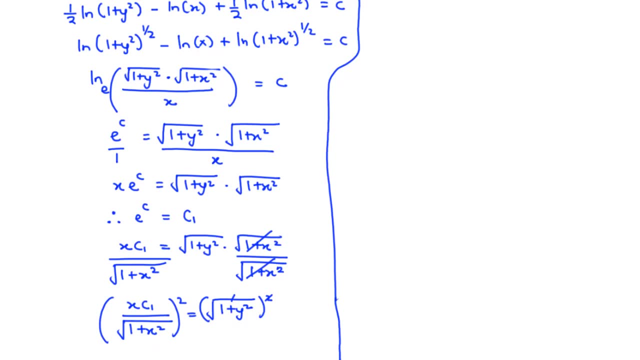 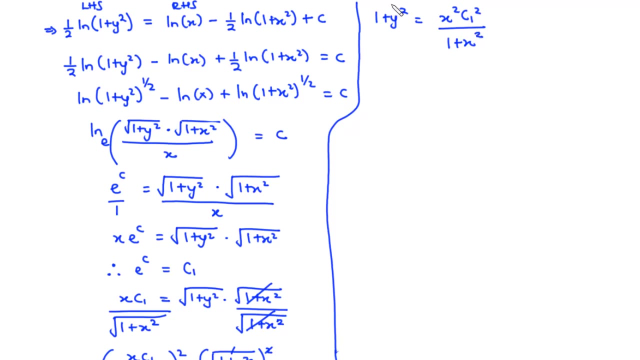 so x squared, c1 squared, all divided by now, here the square cancels the square roots, so we are going to have divided by 1 plus x squared, so 1 plus x squared, and we are going to transpose 1 to the right hand side, so we have y squared equals. 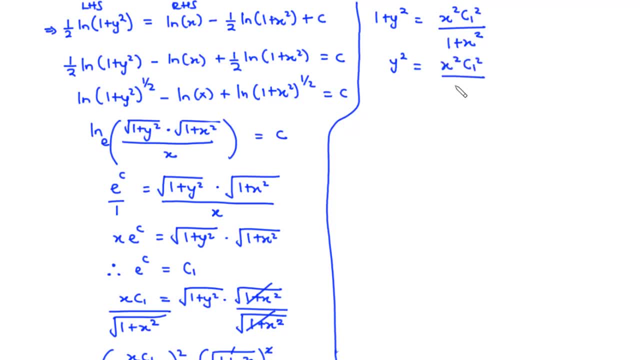 x squared times, c1 squared over 1 plus x squared minus 1. so we take the square root of both sides. square cancels square roots. we are left with: y equals the square root of x squared c1 squared over 1, plus x squared minus 1.. now let's try to simplify this.